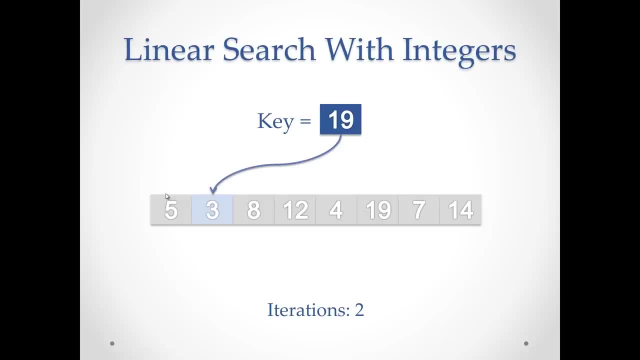 it just moves on to the next element. It's just looking for that key value. So it compares 19 with 3. again, They're not equal, so it just keeps moving on until it finds 19.. So since the function finally found the key value, it just stops and returns the index that it's 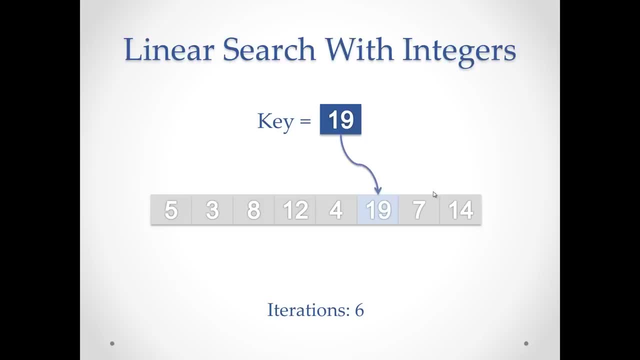 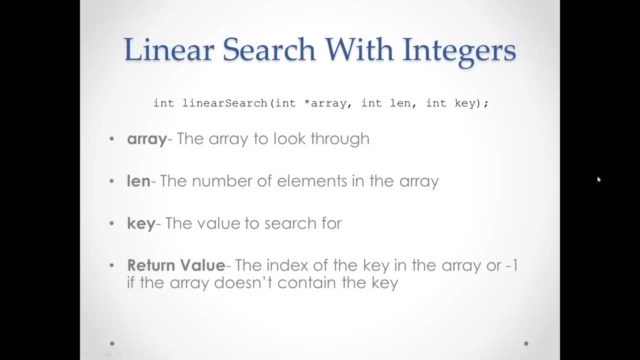 currently at. It's currently at the index of 5, so this function would return 5.. So now let's go ahead and take a look at the function prototype for our linear search algorithm. So this is all that it's going to look like. It's going to return an int which is just 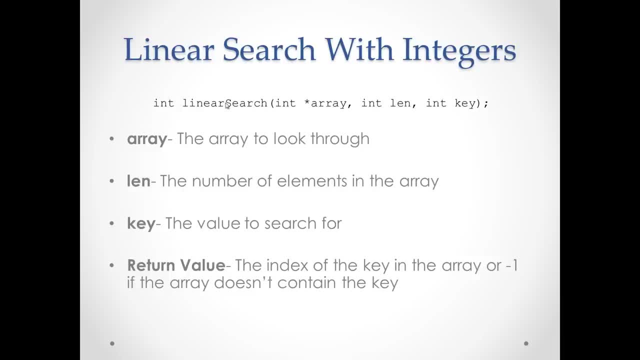 going to be the index of the key inside of the array and we'll just go ahead and call our function linear search. And, like I mentioned before, this function takes three parameters. The first is just going to be the integer array that we're looking through. The second 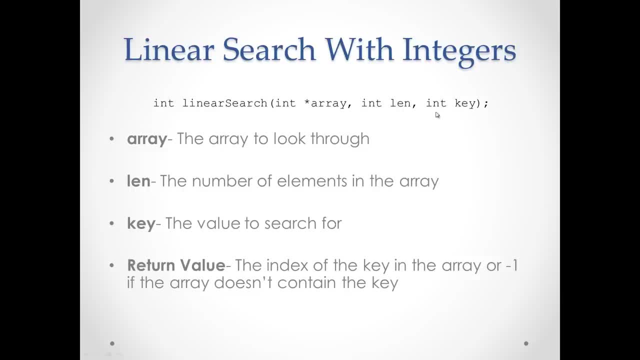 parameter is the length of that array, and the last value is just going to be the key. so the value that we're looking for. And now for the whole function: It's pretty small. So all that this function is going to do is just look through the entire array. It starts at the very beginning of the array. 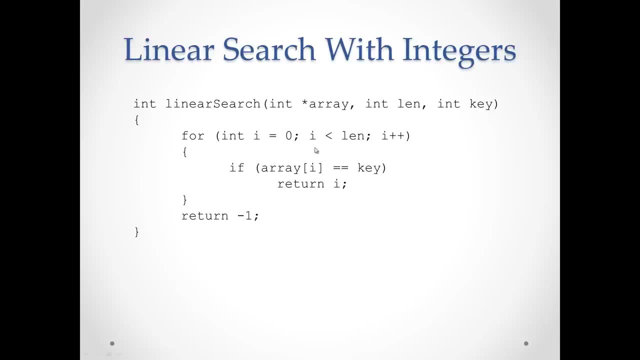 and compares every single value of the array to the key value until it finally finds the key. If it finds the key, then it just returns the index that it's at. If it goes through the entire array without finding the key, then it just returns negative 1, indicating 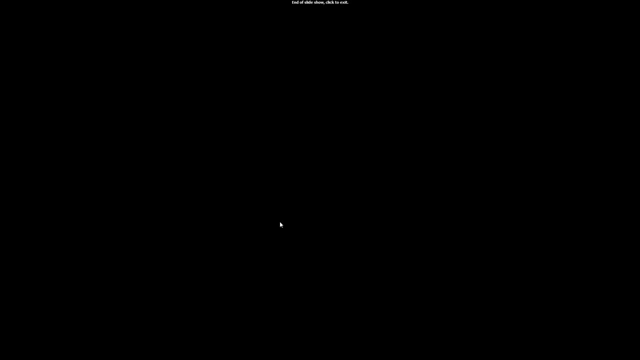 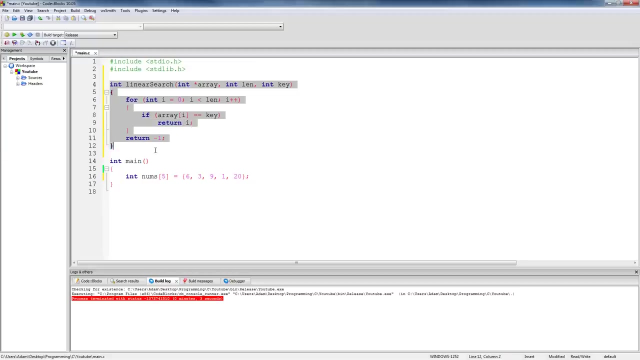 that the key is not inside of the array. So let's just go ahead and go into code blocks here and test out the linear search algorithm. So just here is the function, right here, and we already have an array written out for us. So we'll just go ahead and call the linear search algorithm on this nums array, right? 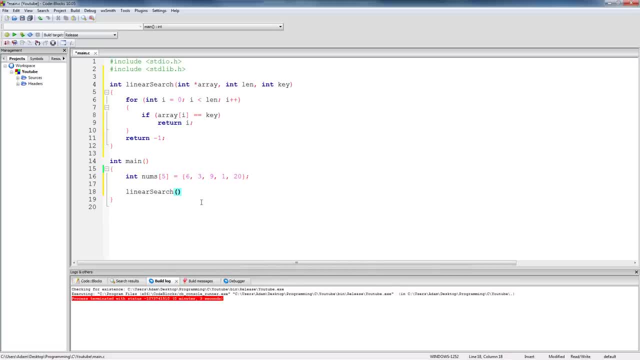 here. So we'll say linear search and we'll pass through nums as the array that we're looking through And the length of the array is 5, since there are 5 elements inside of the array, And then the key value that we're looking for we'll say is 1.. So we're looking 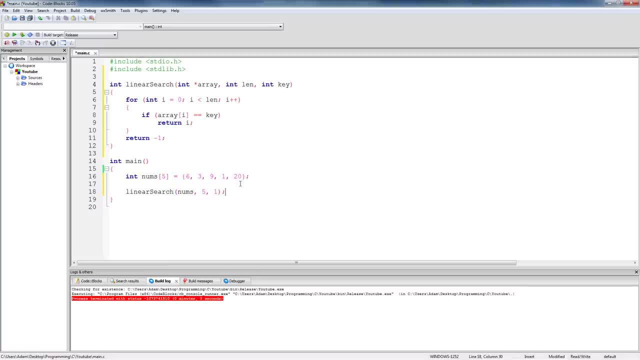 for 1 inside of this array right here, And then we'll just go ahead and print out the return value onto the screen so that we can see what it is. So we'll say printf mod i, since this function returns an integer, so mod i and the line, And then we'll just go ahead and print this out.